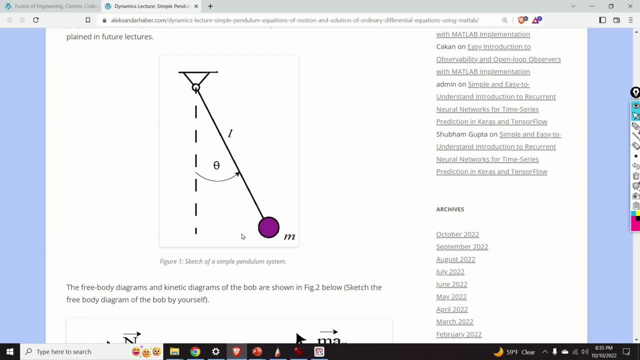 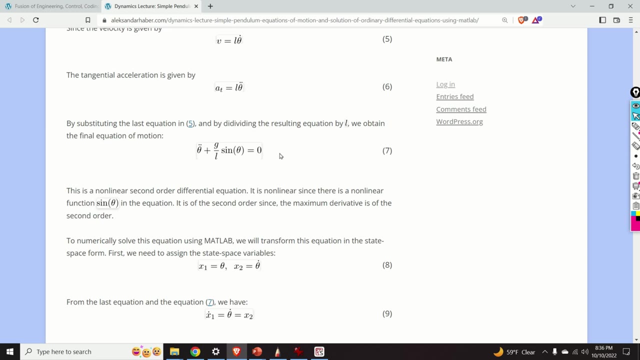 over here. The length of the pendulum is L and here is the mass, m, And the variable that describes the position of the pendulum is given by theta. The ordinary differential equation representing the dynamics of this pendulum is represented by this equation. 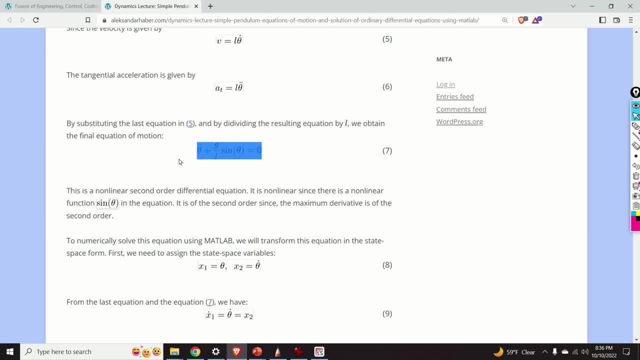 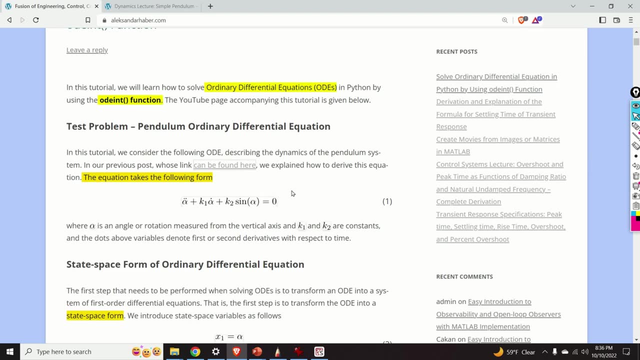 the equation number 7.. The equation number 7 represents the dynamics of the pendulum, and this will be the starting point for my derivations. Now let's go back to our post. Here is the equation 7 in a more general form, where I added over here a damping term. So 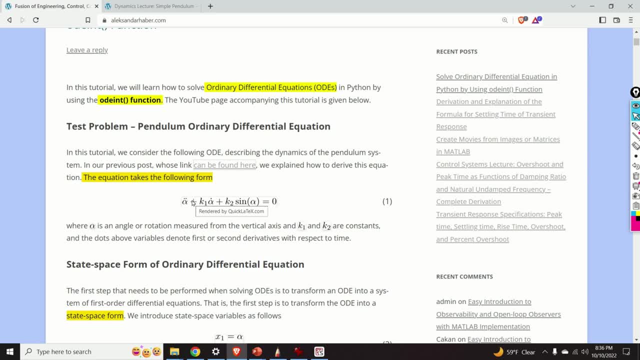 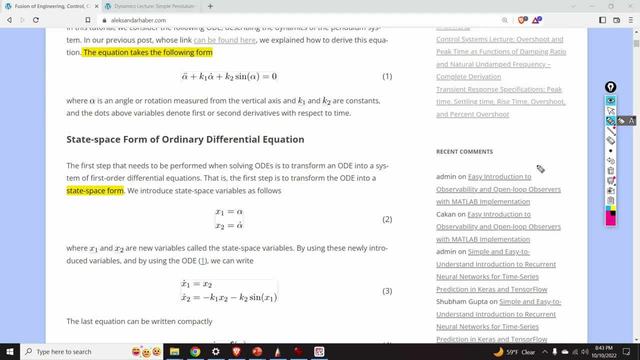 alpha is basically equal to theta. It's the angle of displacement of the pendulum. This alpha dot is basically the first derivative on the pendulum. The position of the pendulum is the constant, and k1 and k2 are the constants, The first step that needs to be performed. 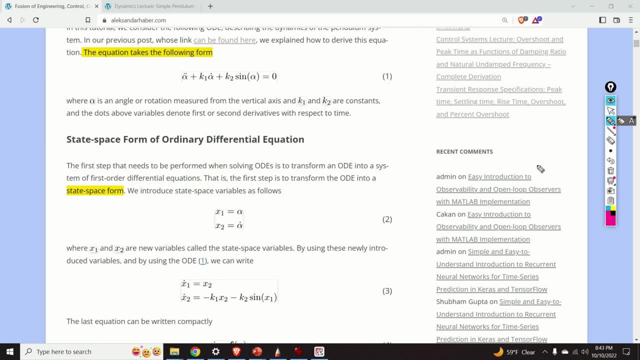 when solving ordinary differential equations is to transform the particular ordinary differential equation that we want to solve into a system of first-order differential equations. Wow, This sounds quite complex, right? Well, this procedure is not complex in practice. Actually, it's very simple. So let us consider our original equation. This is the second-order differential. 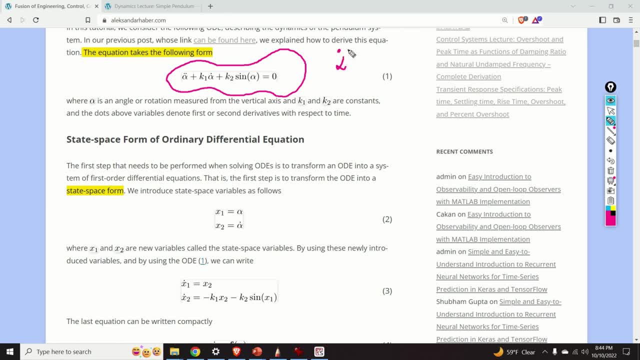 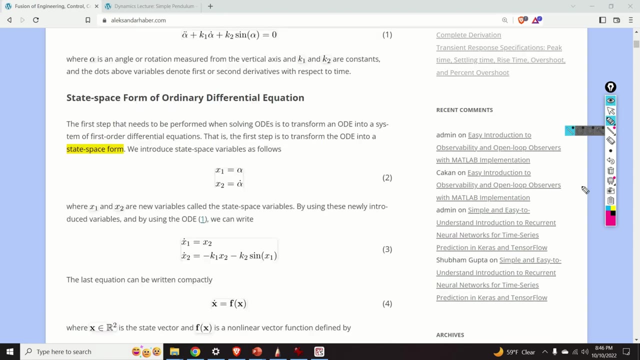 equation because we have alpha 2 dots. Okay, now I'm claiming that this equation can be written as a system of two equations of the first order. Okay, so let's see how to do that. The main idea is to introduce new variables that are called state space variables. So 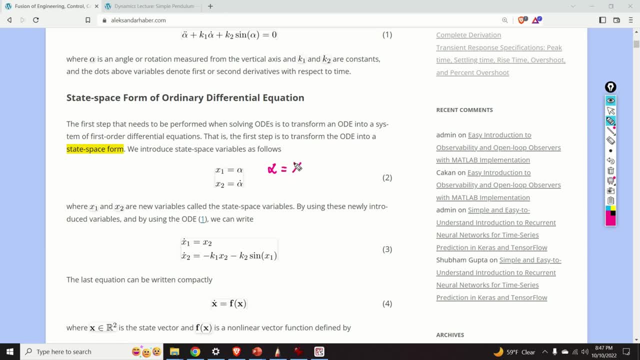 I can write: alpha is equal to x1, where x1 is a new variable that is often called the state space variable, And I can say that alpha dot is equal to x2.. So x1 and x2 are new variables Now. 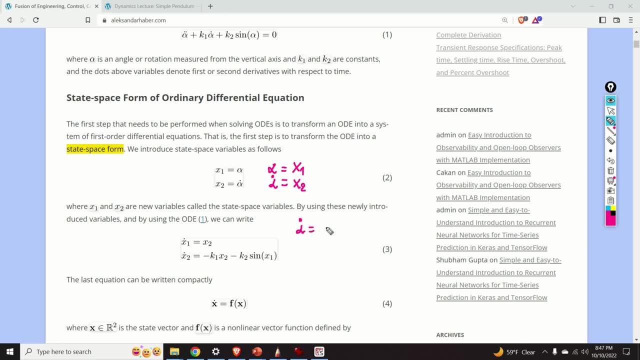 let's differentiate alpha. So we have: alpha: dot is equal to x1 dot and basically x1 dot is actually equal to x2.. So here is my first first-order differential equation. So let us obtain the second one Now. from this equation I can obtain that x2 dot is equal to x1 dot. 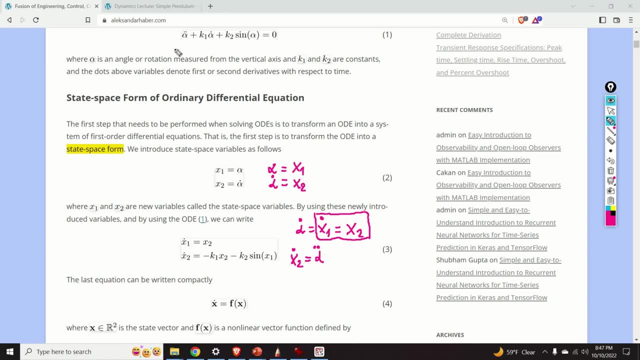 The third then put here: alpha dot is equal to alpha 2 dots And, going back to our original equation, we can write that alpha 2 dot is equal to minus k1, alpha dot minus k2, sinus-alpha, And then, as the result we obtain, this is equal to minus k1, alpha dot is x2,. 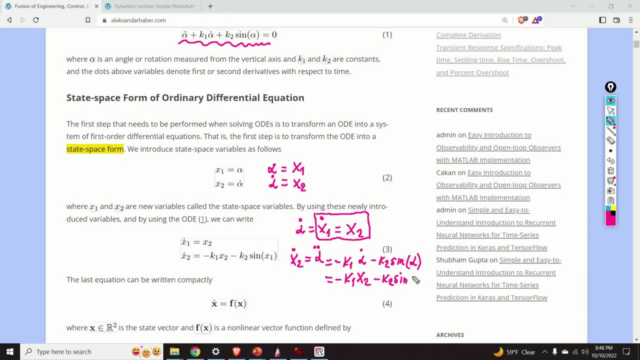 minus k2, sinus-alpha minus x2 dot, And I can say sinus x1. and this is our second equation that's also given over here and this is the first one. so at the end we have transformed the original second order differential equation as a system of two. 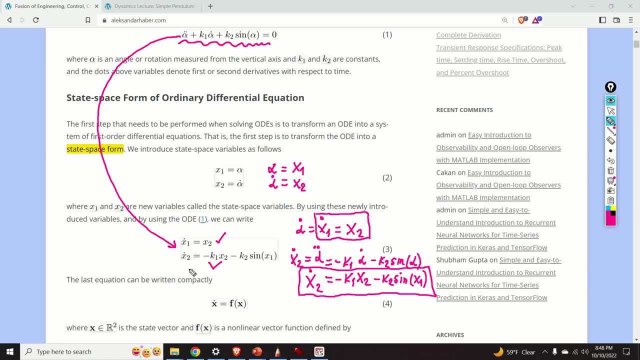 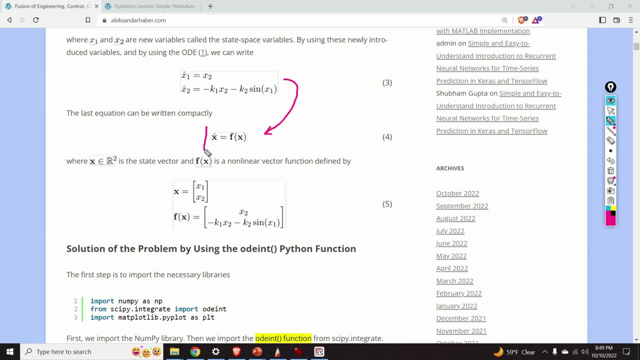 first order, differential equations. now, these two equations can be written in the vector form given by this equation. and here's the vector form. this is the right-hand side of this vector equation, this vector function f of x. ok, now we are ready to code this equation in Python. 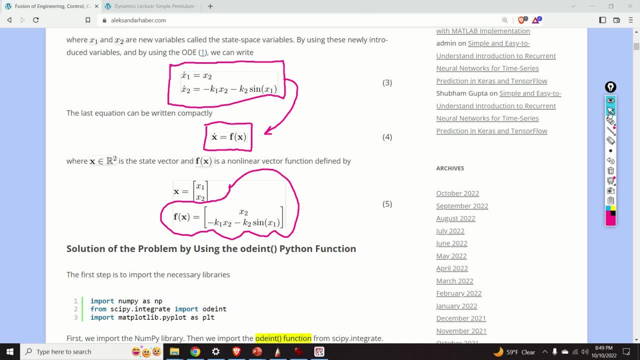 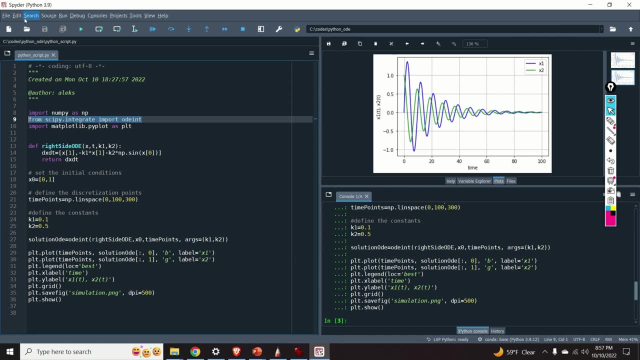 and to solve it. next I will explain the Python code for solving the ordinary differential equation. as you can see, I'm using the spider Python environment in anaconda. ok, so the first step is to import the necessary libraries. first I import the numpy library, since I need 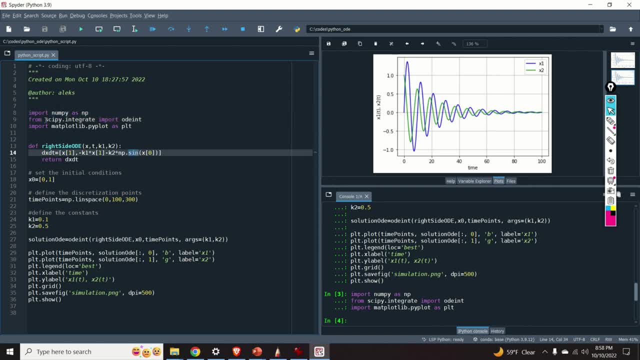 the sinusoidal term over here. then from I import all the int function, so this function will be used to integrate or to solve the ordinary differential equation. then I import the plotting tools. ok, the next step is to define our ordinary differential equation. basically, we define a Python function that is in. 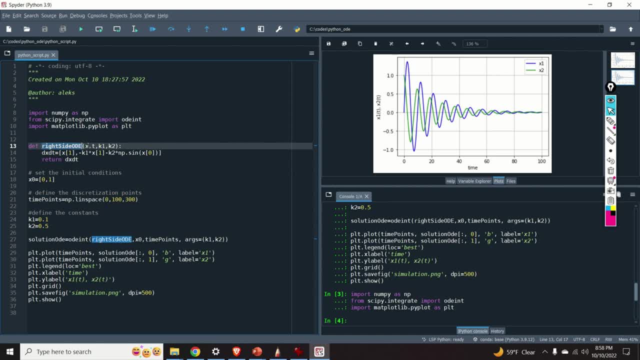 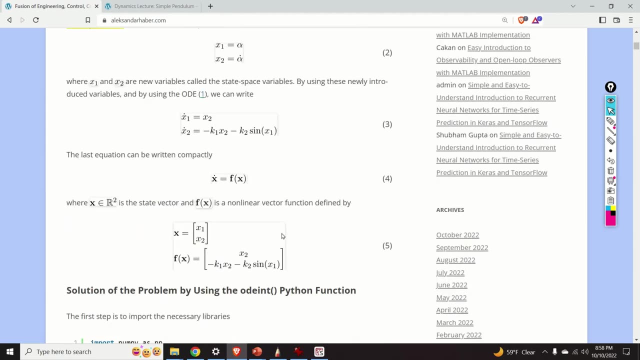 my case called right side ODE, and this function, as the name suggests Suggests, defines the right-hand side of my state space model. So let us go back and let us look at our state space model. So here is the state space model, so we need to write a python function that will: 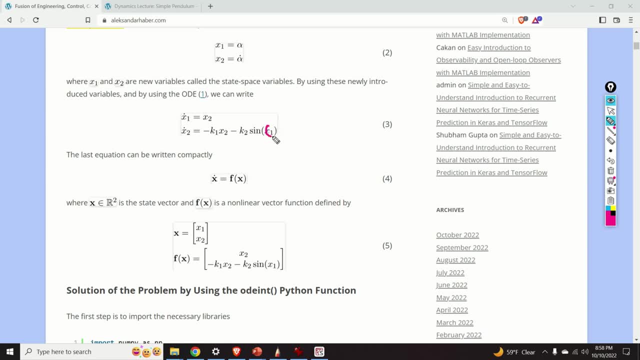 for given values of x1 and x2, evaluate these two quantities, that is, evaluate the complete right-hand side of our state space model, or, Better to say, evaluate this vector. Here is one very important remark: Here I'm using column vectors. however, the function Or the int in python uses the column, uses the row vectors. 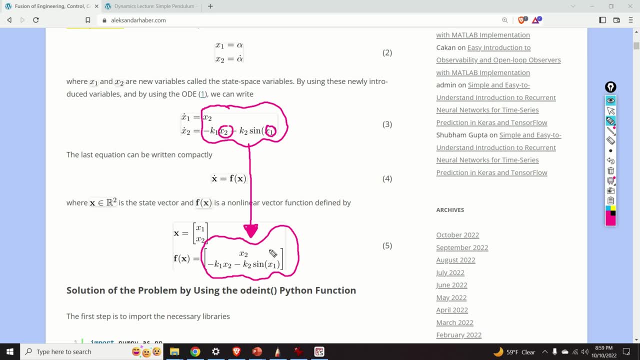 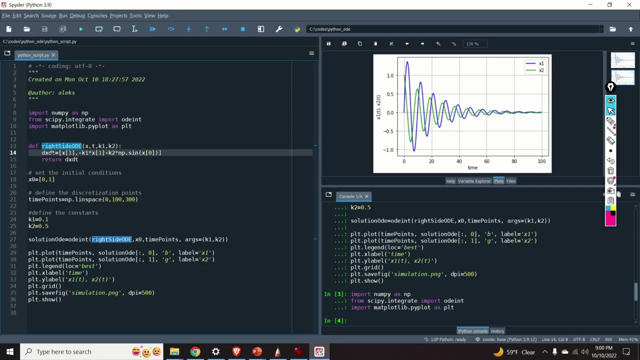 So be careful about that, since in the post there Are column vectors. however, in the code they are basically the row vectors. Okay, let us quickly go back to our python code and let us define the right-hand side. Here is the right-hand side, But before we define the right-hand side, we first need to explain the arguments of this function. 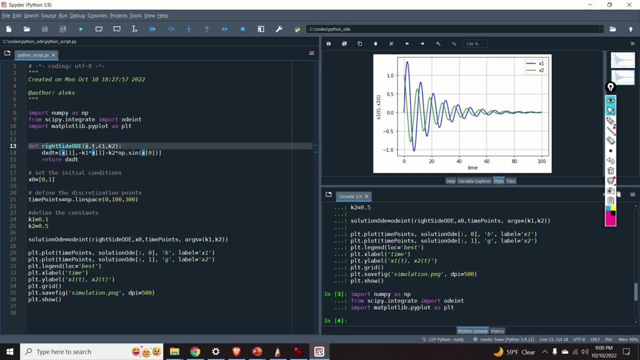 The first argument is the row vector x. this is our dependent variable. the second argument is the time or The independent Variable, and the second, actually the third and fourth arguments are the constants. Here is our right hand side. Basically, the right hand side is the row vector where the first entry is: 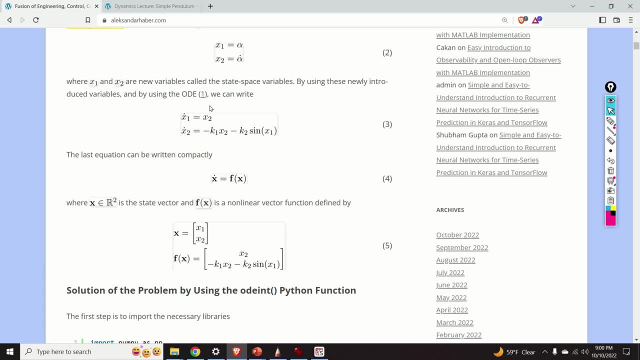 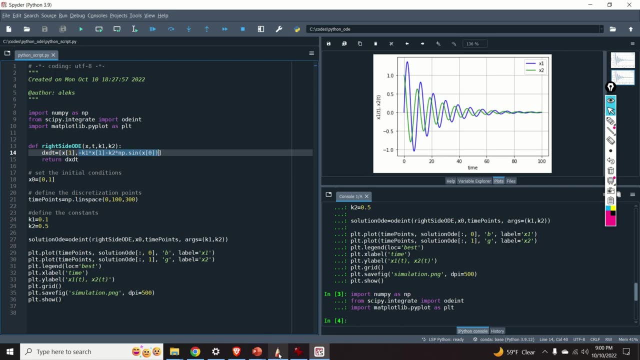 actually defined over here and the second entry is defined over here. here you should be very careful, because the Python programming language indexes the vectors or the matrices starting from 0. so x1 is actually x2 over here and x0 is actually x1. just please keep in mind these things. 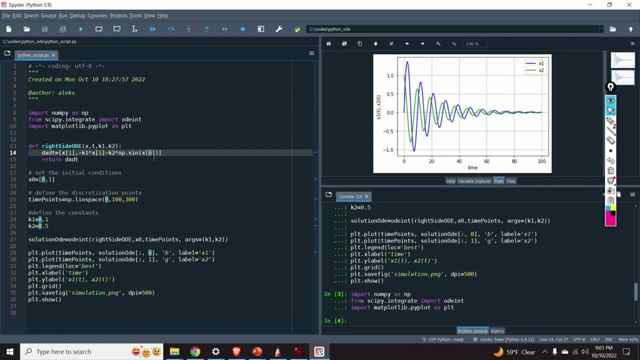 when coding, because many errors happen because people start counting from 1. however, Python is usually counting from 0. and finally, once we have defined the right-hand side, we need to specify the return variable, and this will be this term: dx, dt. that is the first derivative of X. with respect to dt, you can of. 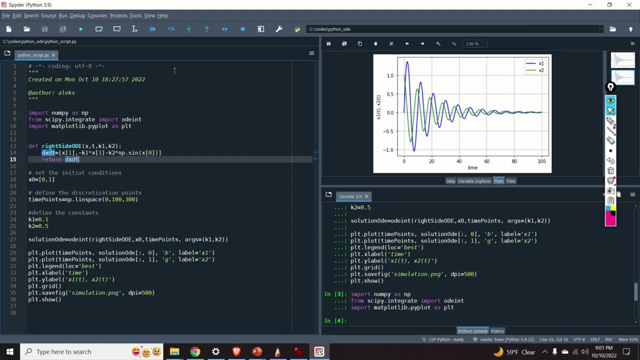 course, use other names for this variable: dx dt. now that we have defined our variable, we are going to define the return variable and we are going to use this term dx dt in our function. we need to define the initial conditions. so here is the vector X 0 that defines the initial conditions. we are assuming that. 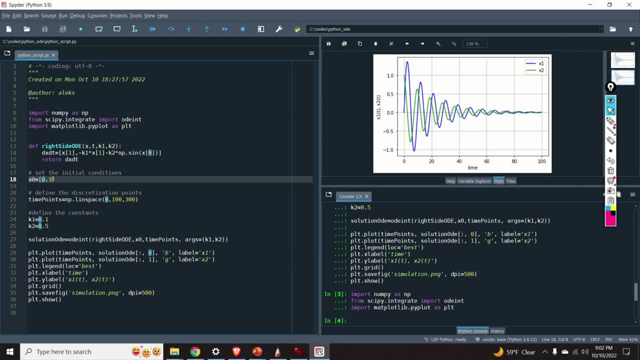 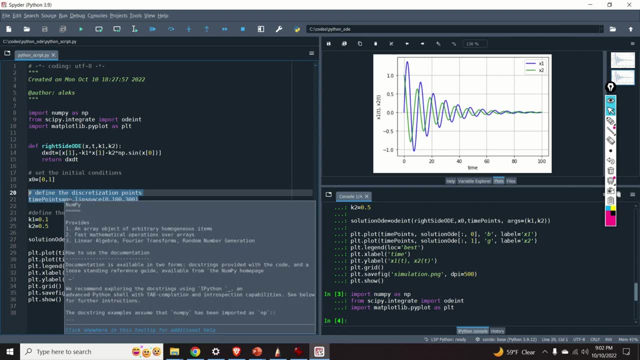 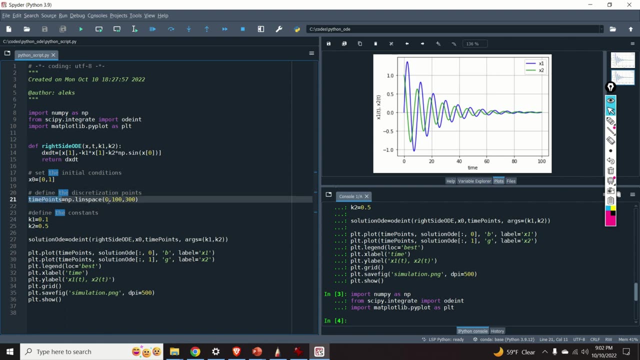 the initial position is 0 and that initial velocity is equal to 1. the next step is to define the discretization points, that is, we define the points at which we will evaluate the solution. these are the time points. so I'm starting from 0, ending at 100 and ending at 100. 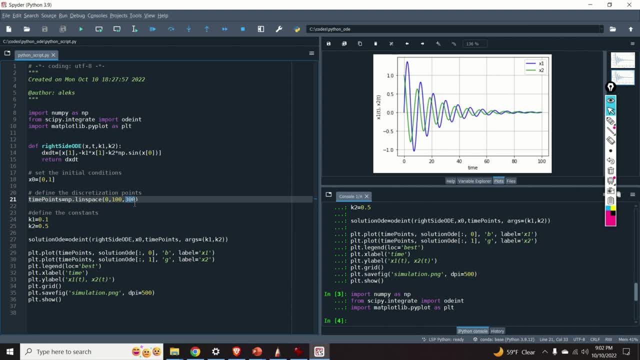 seconds and I'm assuming that I have 300 points uniformly displaced between 0 and 100.. Finally, I define the constants. The constants will be 0.1 and 0.2, and over here I basically call my function odint. The first argument is the function. 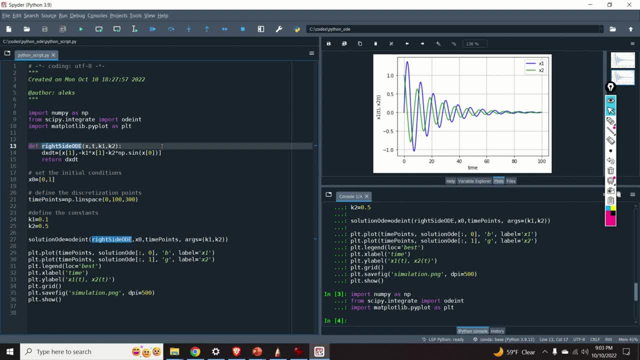 that we have previously defined and that defines the right-hand side. The second argument is the vector- better to say the row vector- of initial conditions. The third argument is a vector containing time points at which the solution will be evaluated, and the final argument is basically a pair containing k1 and k2..